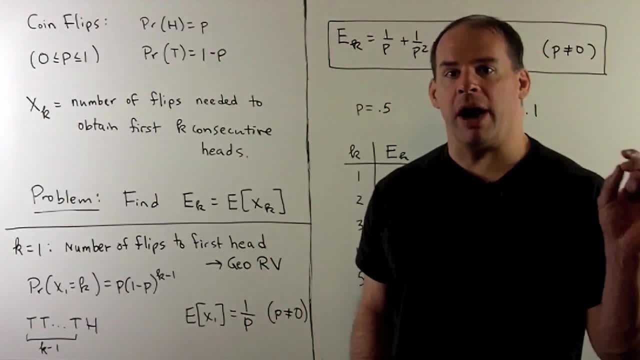 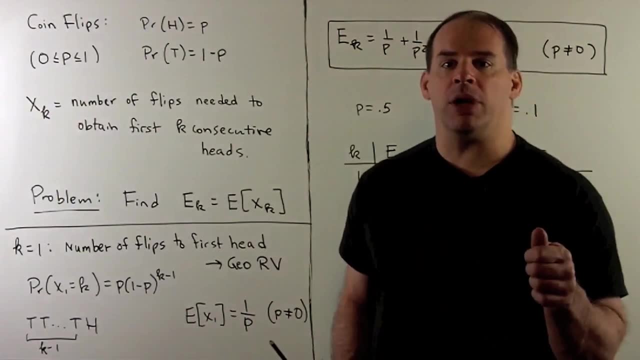 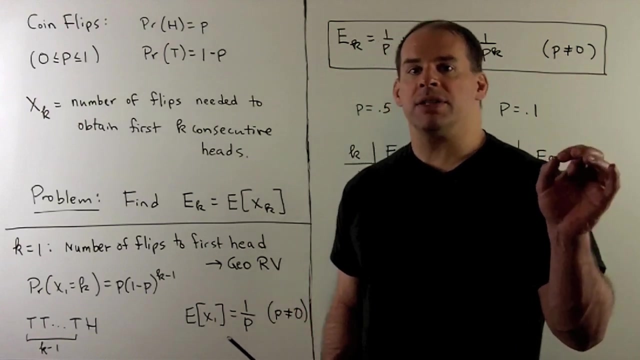 give us the distribution for a geometric random variable. Now, if p is equal to 0,. no matter how many flips we do, we're never going to get a heads. So e of x sub 1 is going to be undefined. Otherwise, the mean of a geometric random variable is just going to be 1 over. 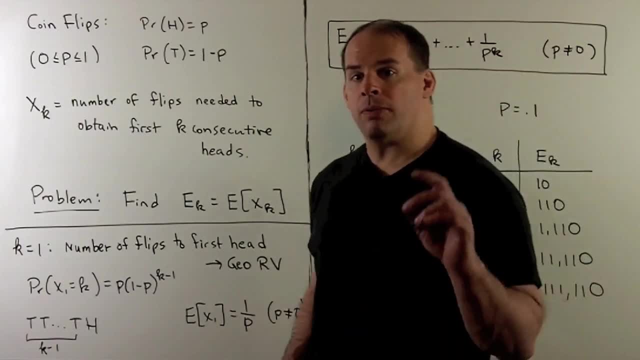 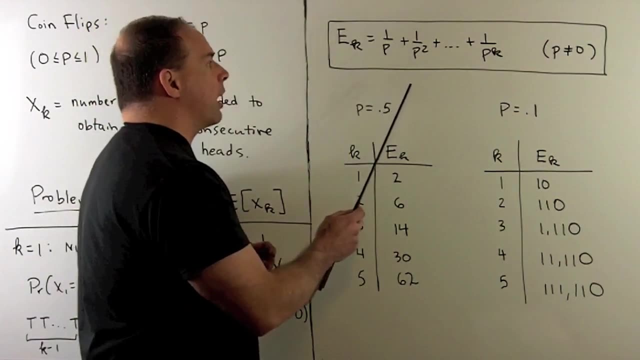 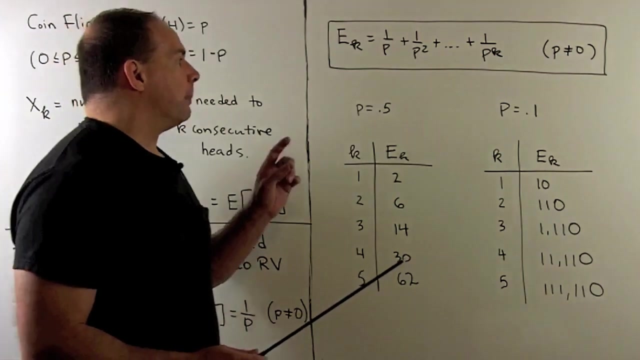 p. For our formula in general, e sub k is going to be given by 1 over p plus 1 over p, squared all the way up through 1 over p of the k, assuming p is non-zero. Now if we consider: 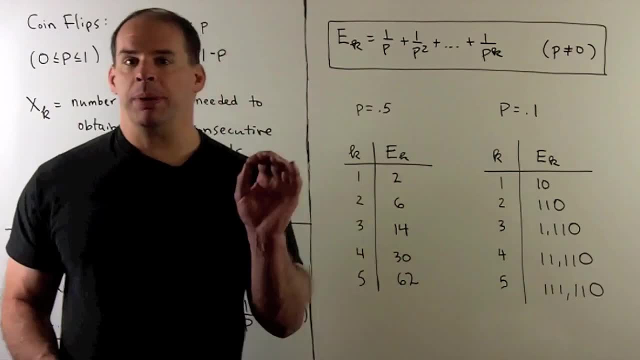 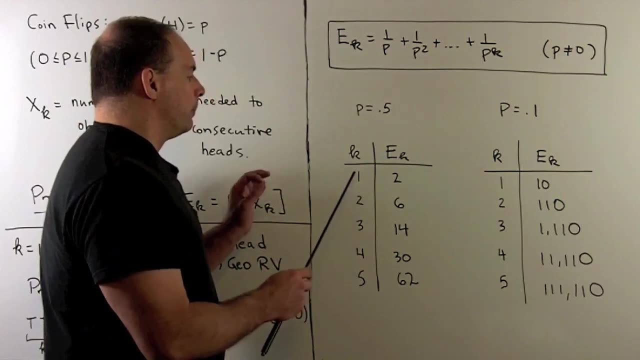 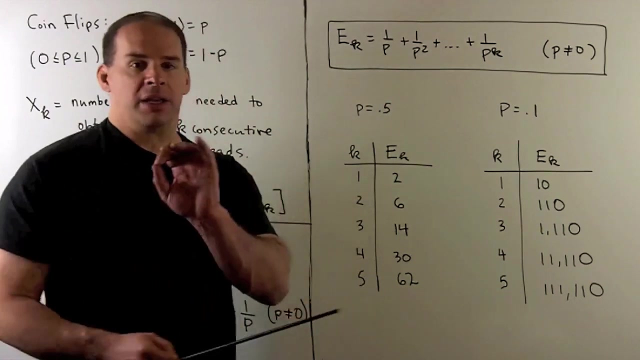 our formula for different values of p. so if I have a fair coin, p is equal to a half and we get the following table. So this is our length. We have our consecutive run of heads. We note as I move to get a consecutive run. 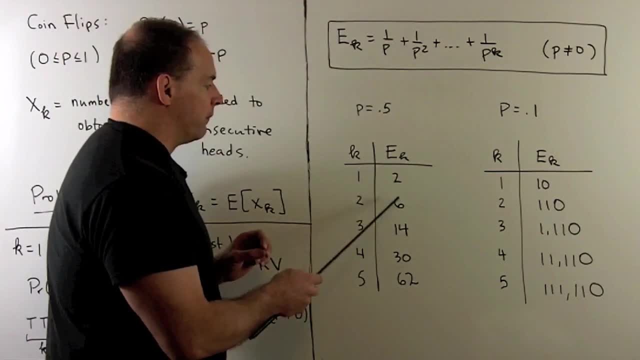 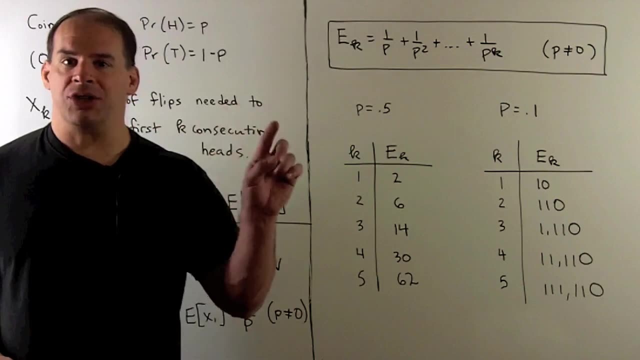 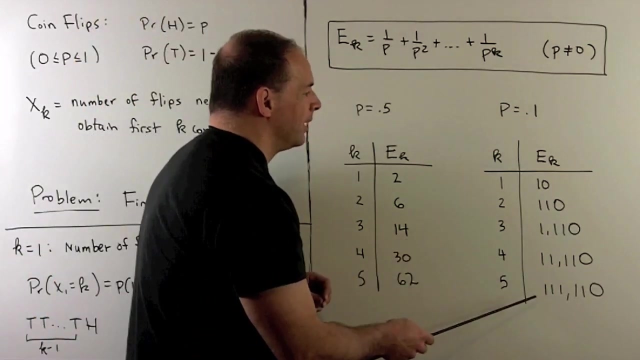 one longer. we're roughly doubling the number that we had from before. When our heads appear less often. so, for instance, if I have p equal to 0.1, we note: okay, we have the following table In this case. as we go down our list, things are growing by. 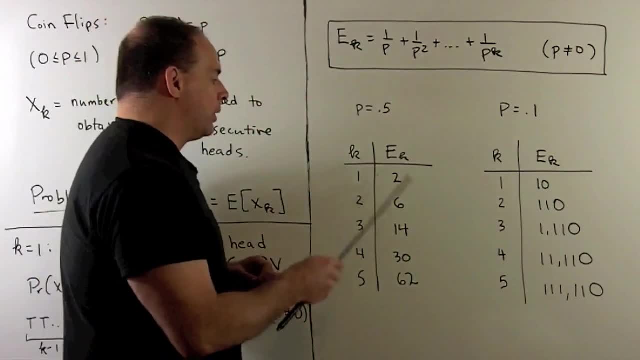 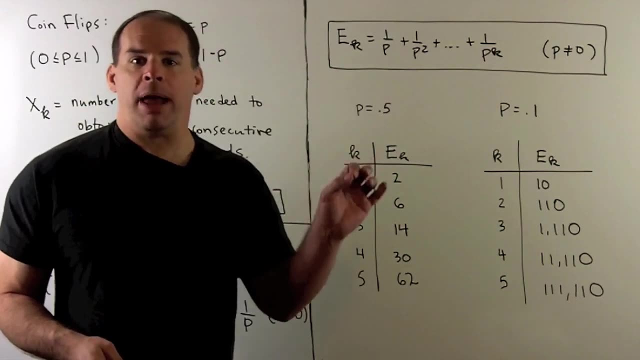 an order of magnitude. So here we're roughly multiplying by 2.. Here we're roughly multiplying by 10.. Okay, in general, roughly you're going to multiply by 1 over p. That's going to be because the 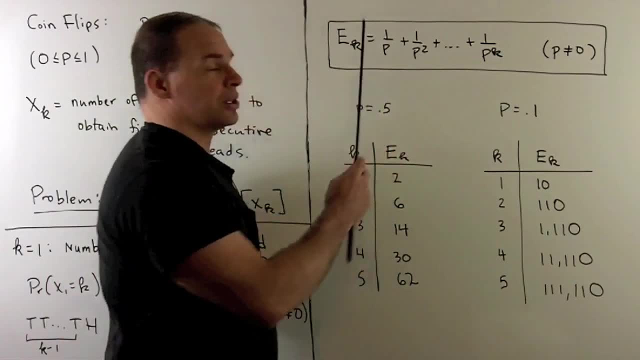 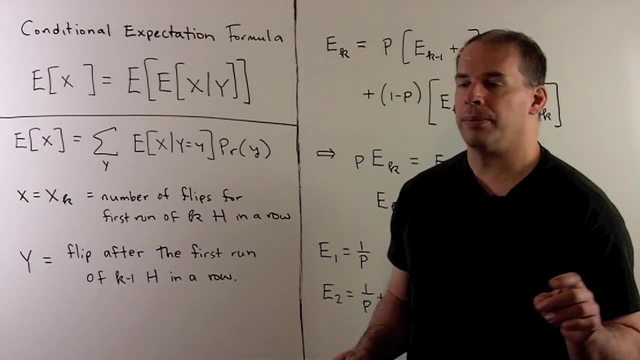 1 over p of the k term is going to dominate all the rest of the terms. Now what does the conditional expectation formula say? I want to compute the expected value of the random variable x. I compute the expected value of the random variable x. I compute the expected value of. 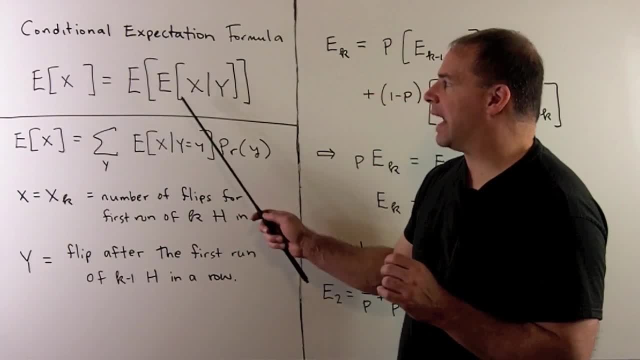 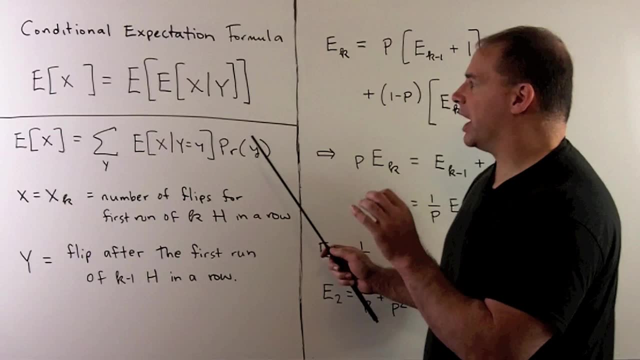 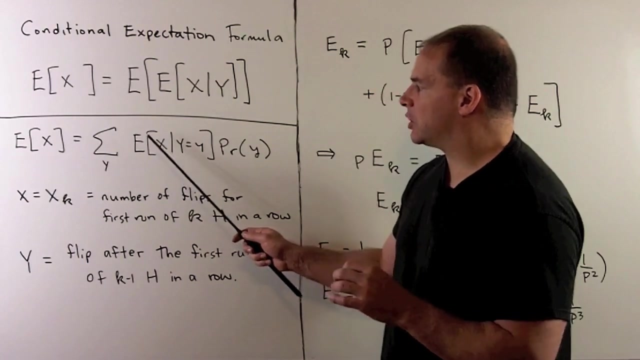 the random variable y, I compute the expected value of the random variable x. Now this is notation. What it really says is: we're going to consider all values that y can take. We sum, We consider the expected value of x conditioned on our random variable. 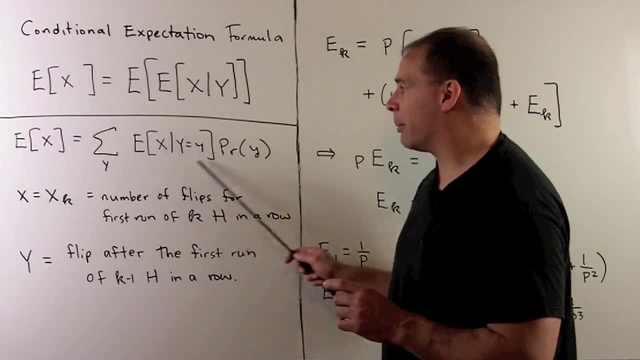 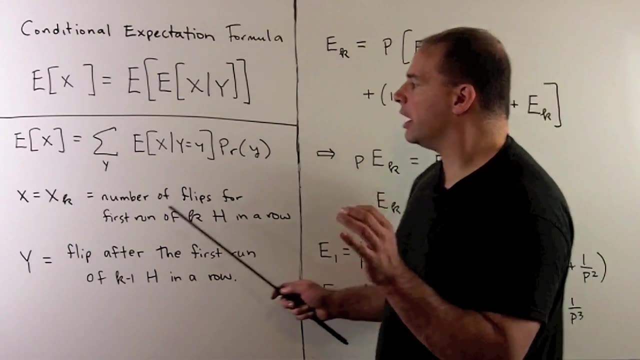 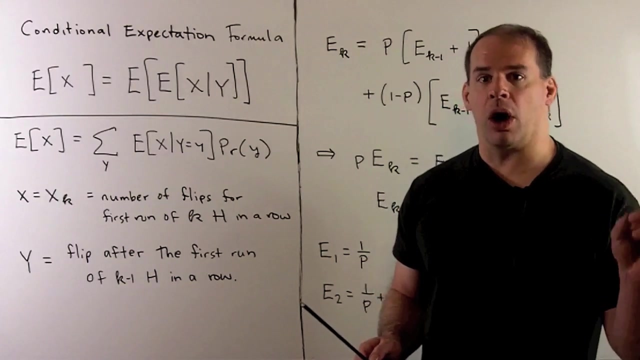 y equal to our given value of y. So this is going to be our number And we wait with the probability of our little y occurring Now. in our case, our x is going to be x sub k. okay, the number of flips to get to our first run of k heads in a row. 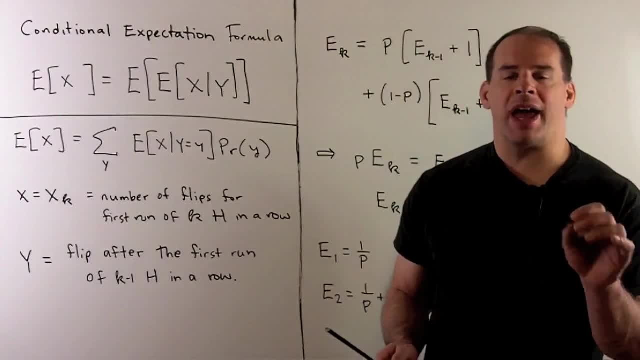 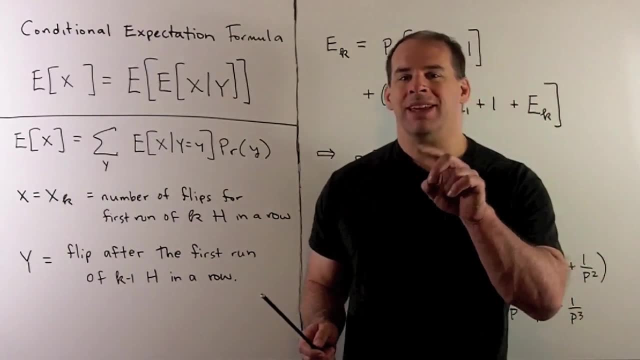 Our y is going to be the flip that occurs after our first run of k minus 1 heads in a row. So note that flip that happens afterwards. if it's a heads, we have what we want: k heads in a row. 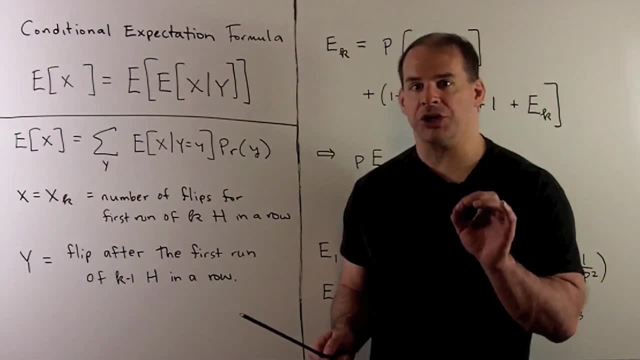 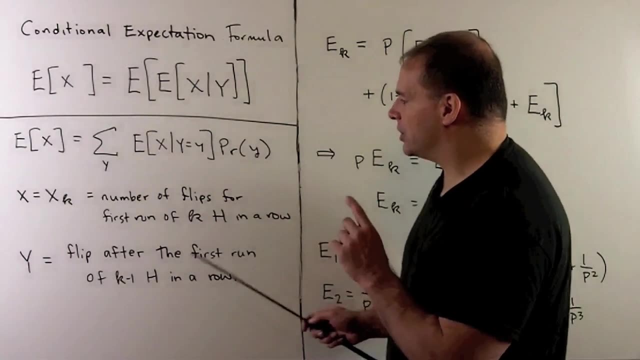 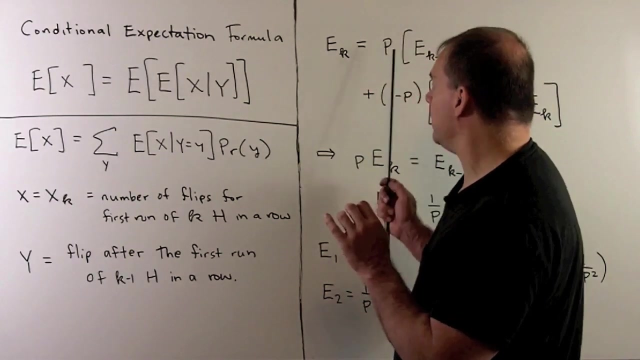 If we get a tails, then we just got to start over from scratch. Now let's take a look at the formula. So if we get a heads in this flip after the first k minus 1 heads in a row, the probability of that's going to be p. 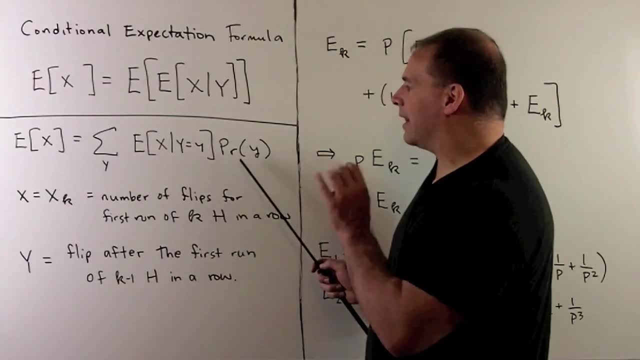 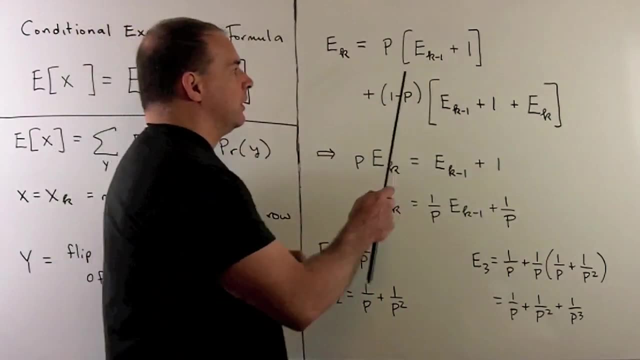 What about the expected number of flips, given that that last one is going to be a heads? Well, we're getting our k heads in a row, so the expected number of flips that we need will be the expected number to get k minus 1 in a row. 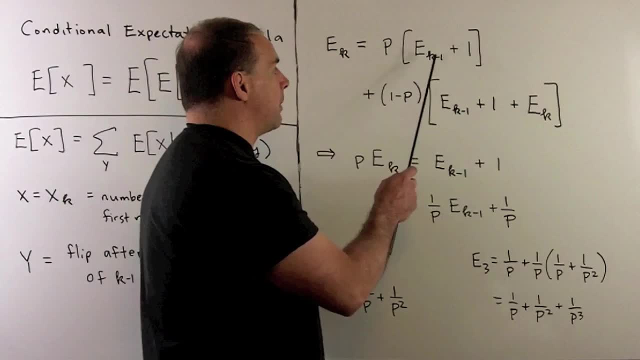 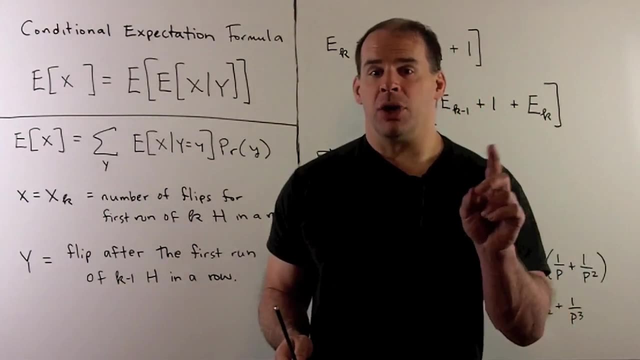 And I just have to add 1.. So e to the k minus 1 plus 1.. What happens if that flip is a tails? Well then we reset. So the idea is that tails is not going to help us build k heads in a row. 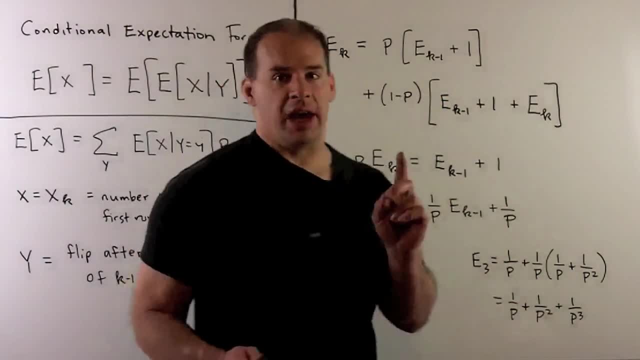 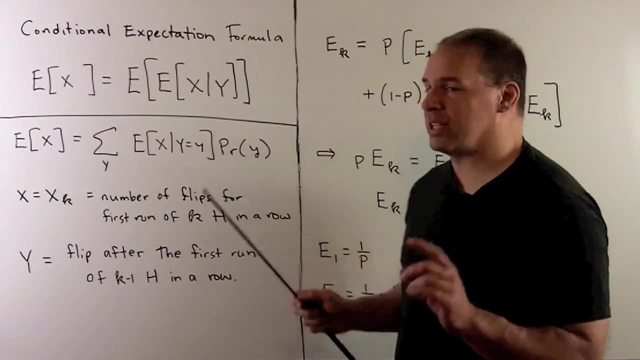 So we're going to have 1 minus p for our tails, Then the expected number that we need to get k heads in a row. given that that was a tails, well, it takes us the expected number of flips to get tails. 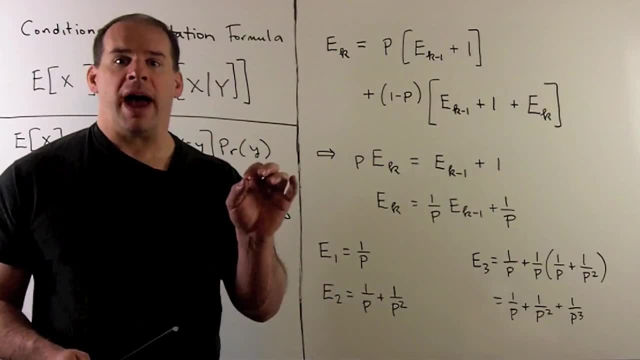 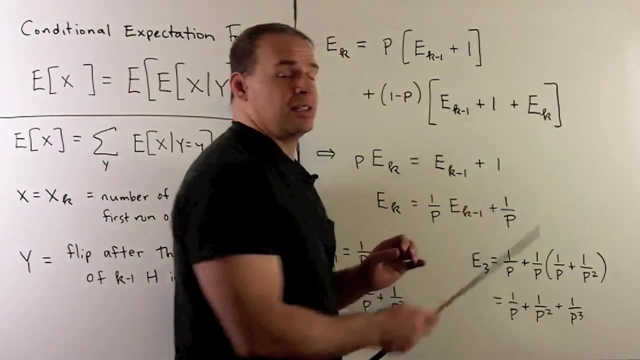 So if we get the k minus 1 heads in a row to get where we're at, we add 1 for the tails And then, since we're starting over, we're just going to have to add on the expected number of flips to get k heads in a row. 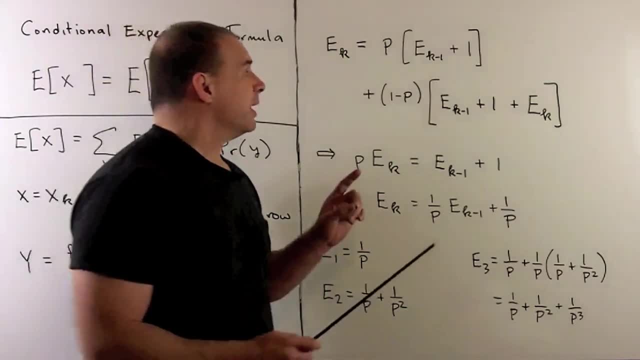 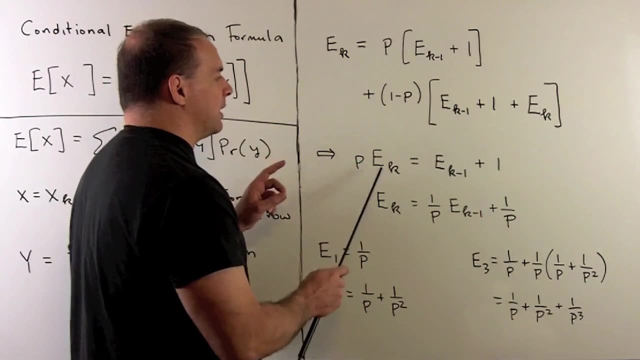 That's just starting from scratch. So this is going to give us our formula. Now, if I clean this up, okay, I'm going to have p, e sub k equals e sub k minus 1 plus 1.. If I divide by p, we get our recursive formula here.